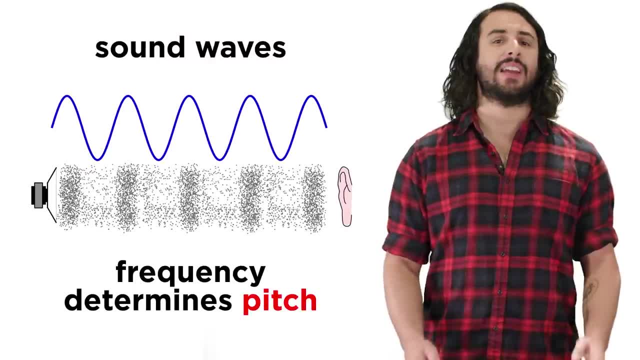 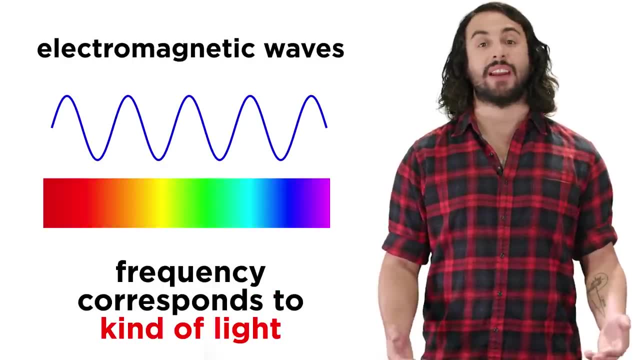 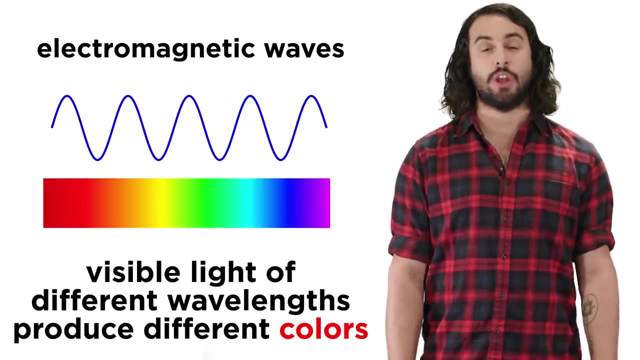 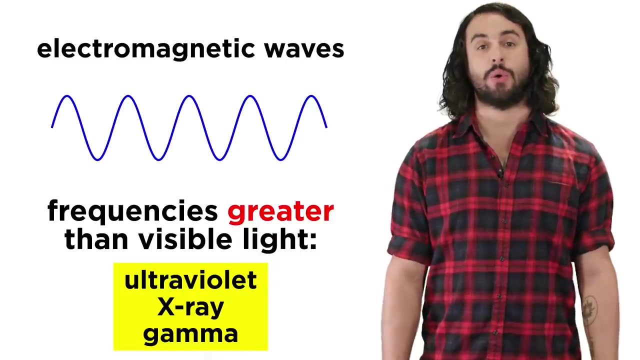 wavelengths and frequencies, But instead of different frequencies producing different pitches, like sound waves, different frequencies of electromagnetic waves produce different kinds of light. If the light is visible, these frequencies will correspond to different colors. Frequencies greater than this will exist as UV radiation, X-rays or gamma rays, and 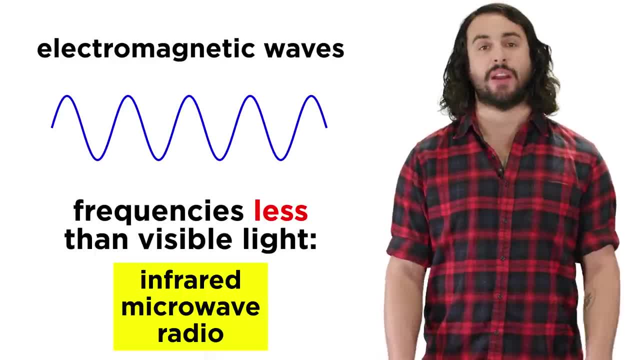 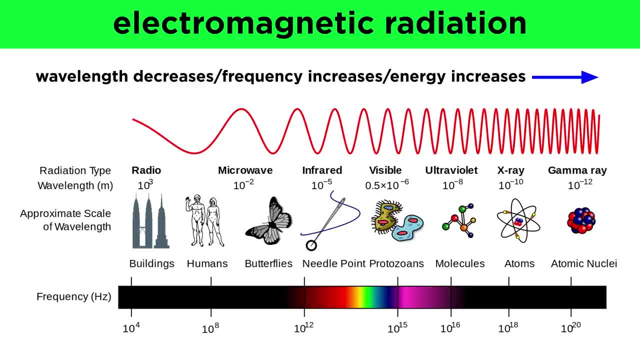 frequencies less than this qualify as infrared radiation, microwaves or radio waves. All of these phenomena are collectively referred to as electromagnetic radiation, and they can be found on the electromagnetic spectrum. Here we can see all the wavelengths and frequencies, ranging from radio waves to gamma rays, and 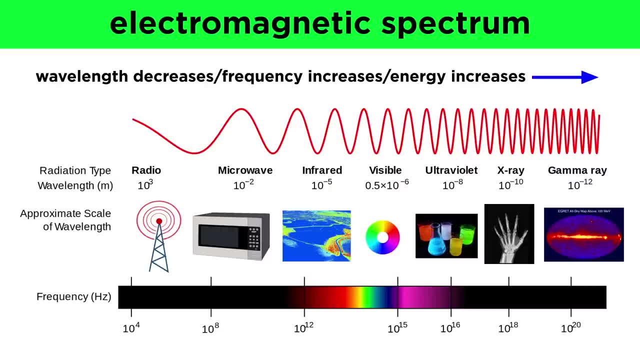 we have found some technological differences. This is because these wavelengths are the most important technological use for all of these in modern society. Even though they seem dramatically different, some requiring things like antennas or other equipment to manipulate all of them are fundamentally the same thing as the light. 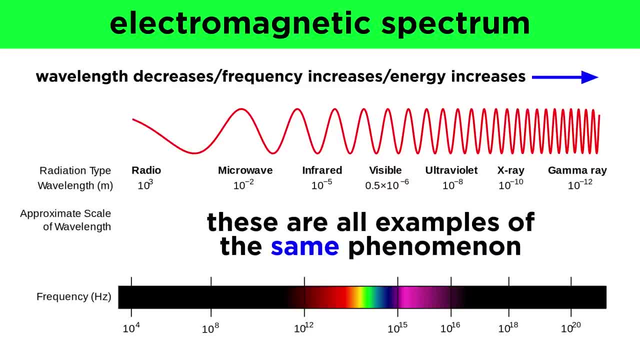 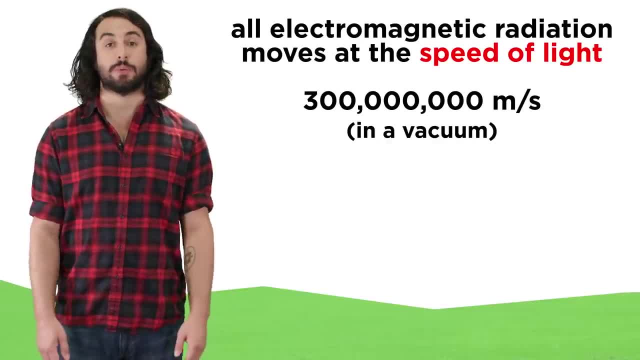 you can see with your eyeballs. They are just of different wavelengths. All electromagnetic radiation moves at the speed of light, which is about 300 million meters per second, in a vacuum- the fastest speed possible in the universe. All electromagnetic radiation moves at the speed of light, which is about 300 million. 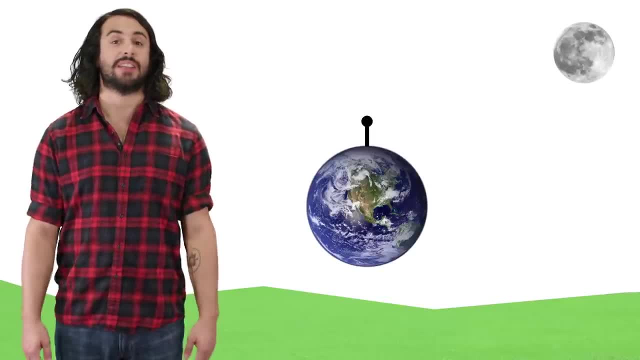 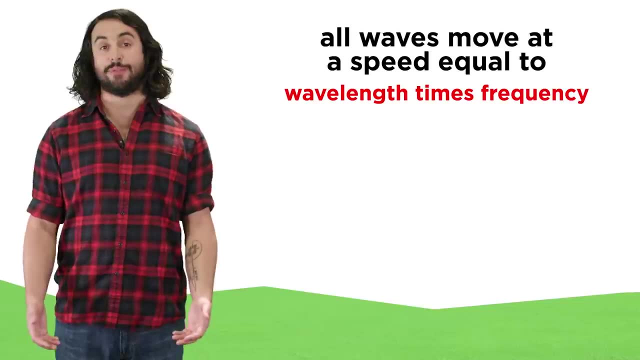 meters per second in a vacuum, the fastest speed possible in the universe. This is fast enough to get from here to the moon in about a second, and since we know that all waves move at a speed that is equal to their wavelength times their frequency, 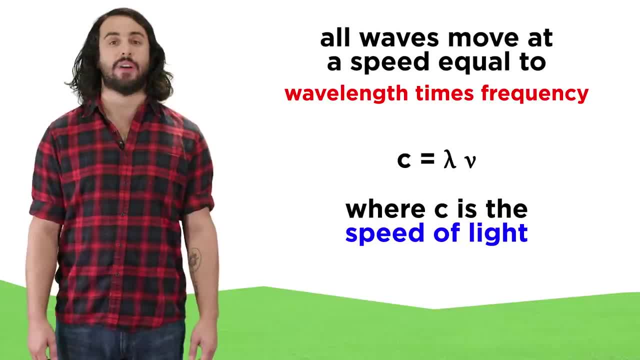 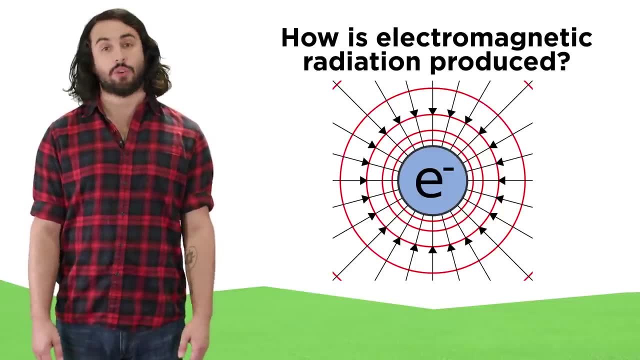 this product will be equal to the speed of light for any type of electromagnetic radiation. How is it that electromagnetic radiation is produced? To answer this question, we have to learn about electric fields, which are coming up soon. For now, let's check comprehension. 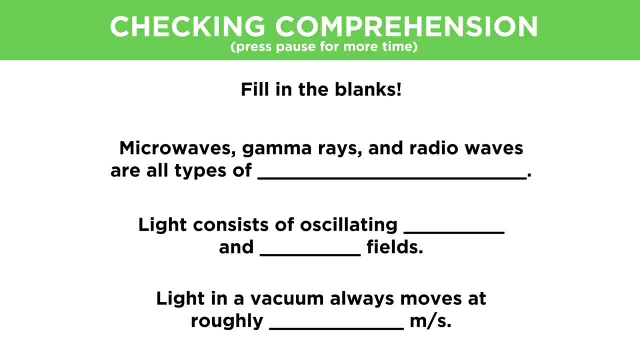 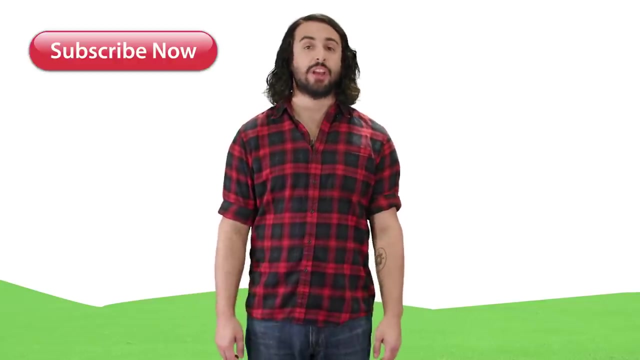 Thanks for watching and I'll see you in the next video. Thanks for watching, guys. subscribe to my channel for more tutorials, support me on patreon so I can keep making content and, as always, feel free to email me. professordavexplains. at gmail dot com.